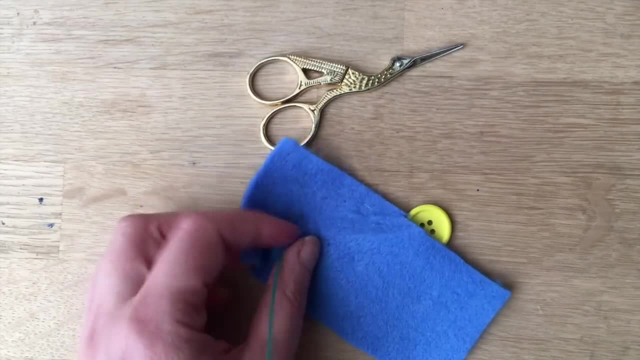 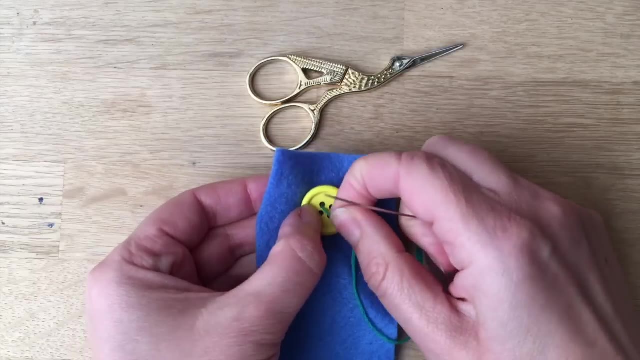 Pull it through. The knot is now holding my thread in place and now it's time to sew on my button. Now most buttons have got four holes, like this one. Some of them only have two, but with four it's quite nice to go across and then across to make like a little X. 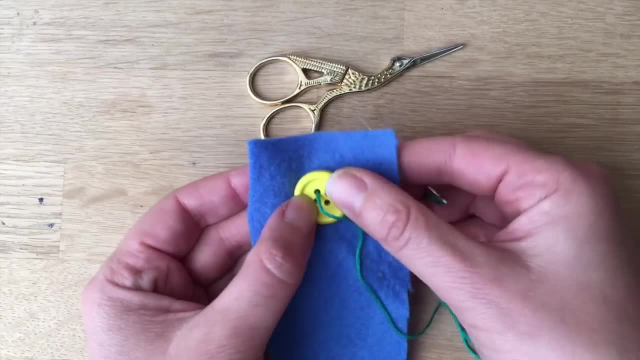 But if you want, you can actually go and make two little neat lines as well. But I'm going to do a little X today. So you've got the button on, now you go to the opposite hole and you push through to the back. 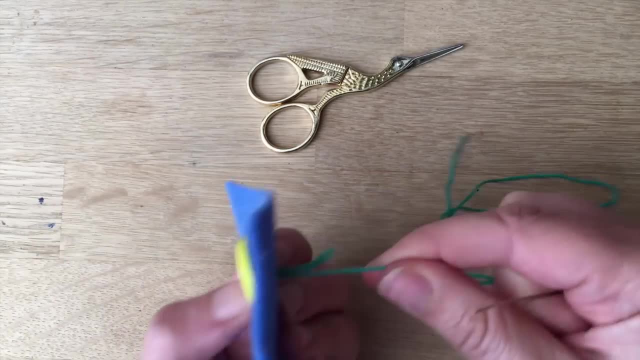 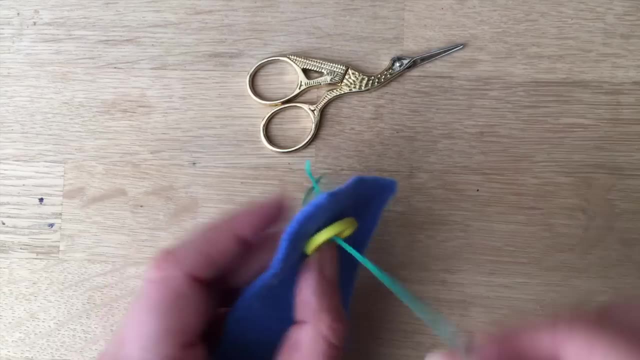 And make sure it's all tied. So I've got the first stitch in place. Now you repeat that two, three, maybe four times. It depends a little bit on your thread and how thick it is. This one's quite thick, so twice will be enough. 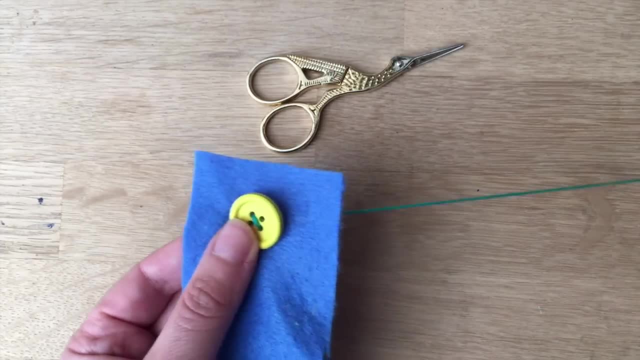 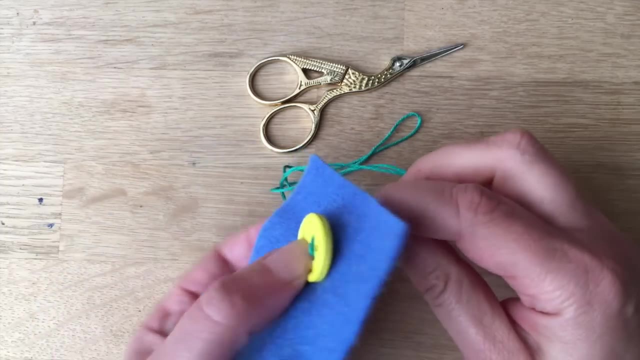 But I think doing it three times is good. Okay, So now I've got twice. So the next thing you need to do is, with the needle at the back, you need to kind of wiggle, wiggle, wiggle until you find the hole, like so, and push it through. 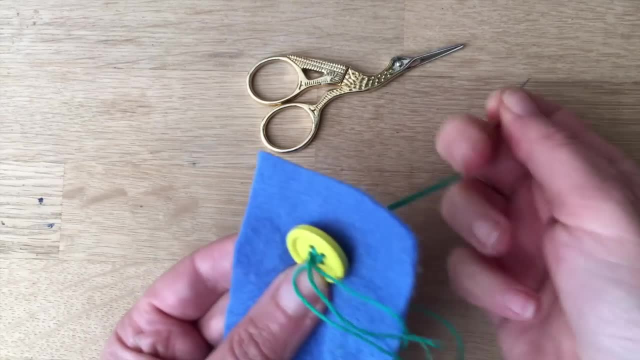 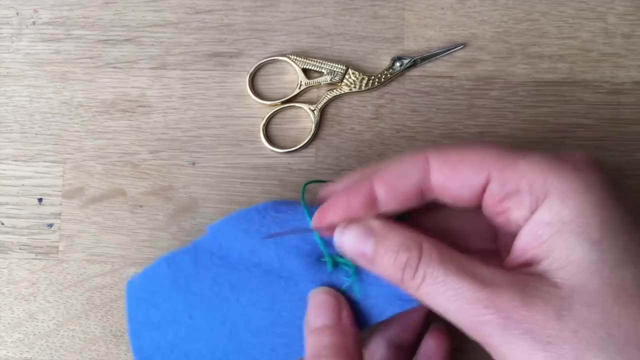 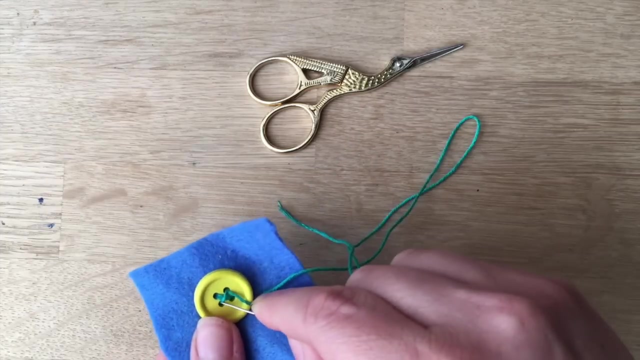 And then you go opposite, push it through and pull it tight. Okay, So again you're going from the back. I can't see it so well from that side. let's do it this side. You go in from the back, you try and find the hole, wiggle, wiggle until you've got the hole, and then you pull it through and round like so. 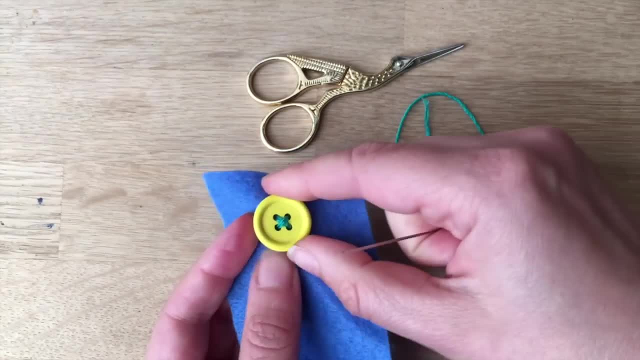 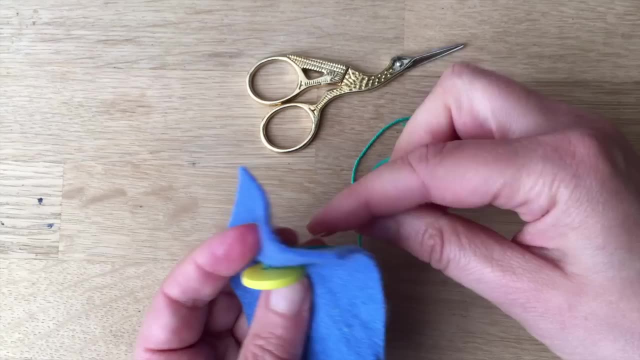 So that's the basic knot sewing off on your button. But what you want is, when you have a button on you, obviously it has a tiny like millimeter away from the side of the fabric And that's so it's easier to knot things, you know, to close your button and have the fabric sit in place neatly without ripping the thread. 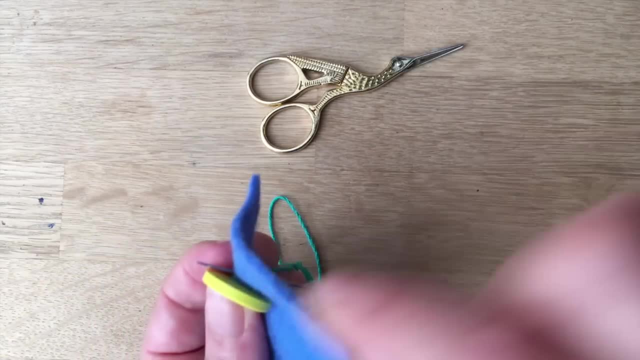 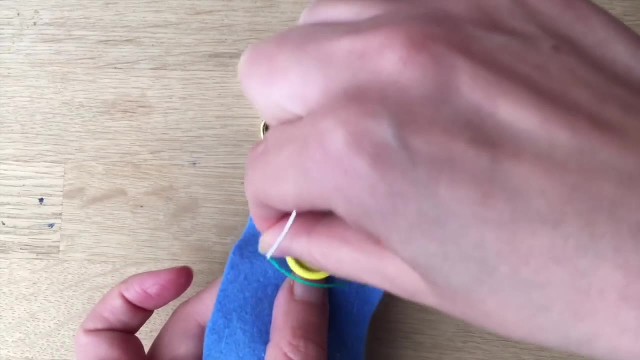 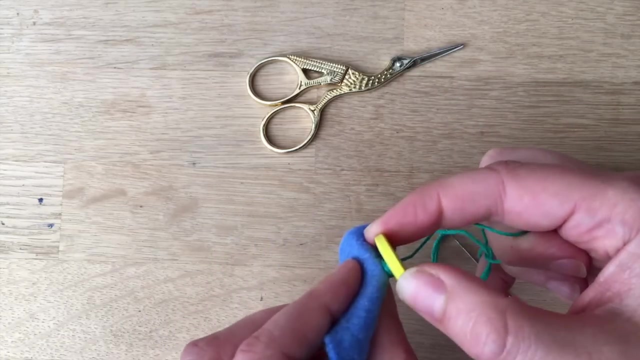 So what you do now is you take your thread and you push it through behind the button, like so, And then you wrap it round once, twice, oopsie, And Three times. Now what that does is it raises it a little bit but also really secures your thread. 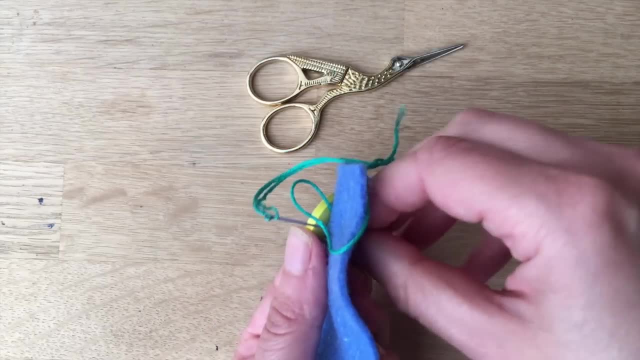 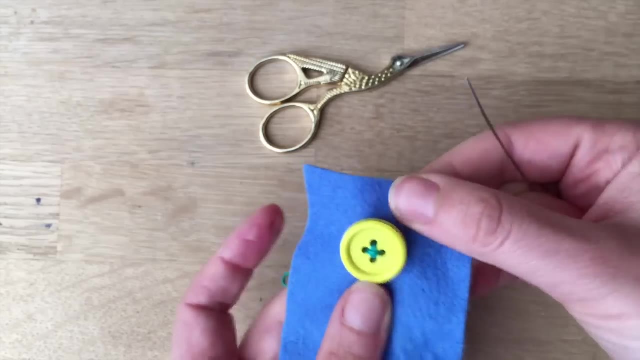 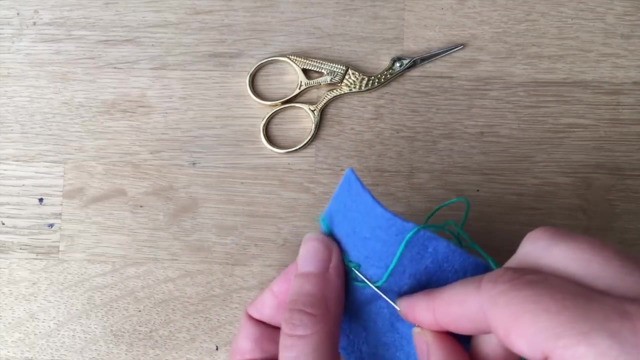 Then you go in, push the needle back to the back, like so Okay, And then it's time to kind of cast off your stitch, So to secure it, get your needle. you find one of your old stitches, so like this one.